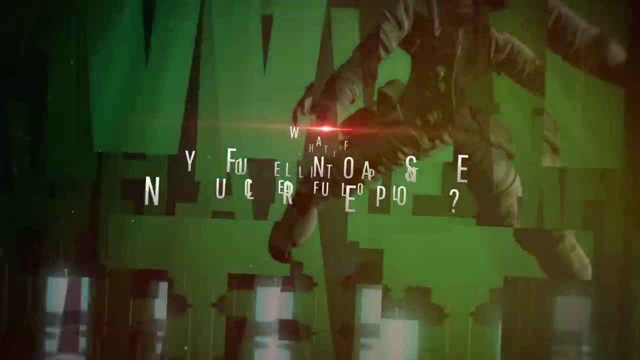 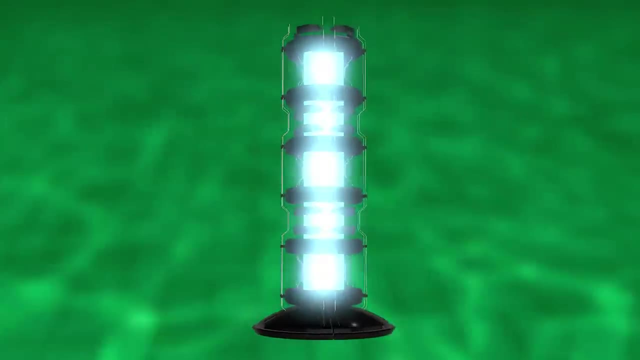 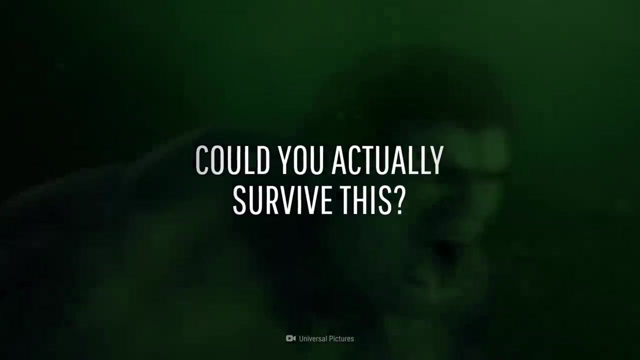 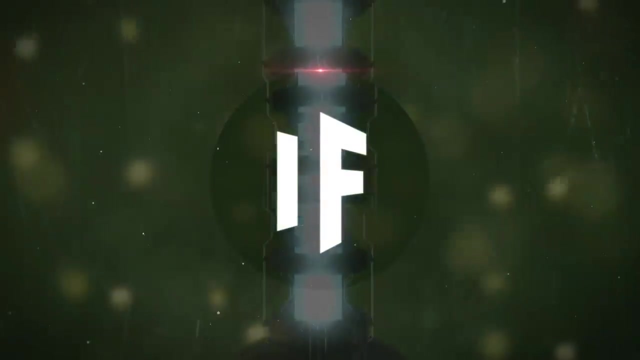 Uh-oh, You just fell into a pool with this thing. What is this? How would falling in here affect your health And could you actually survive this? This is WHAT IF, and here's what would happen if you fell into a pool full of spent nuclear fuel rods. 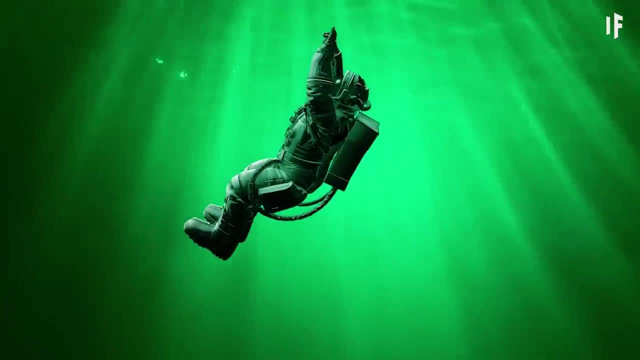 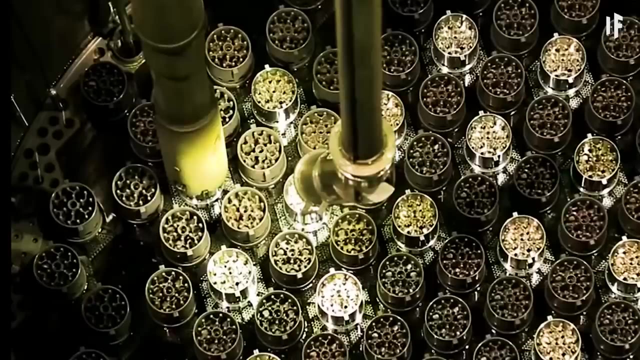 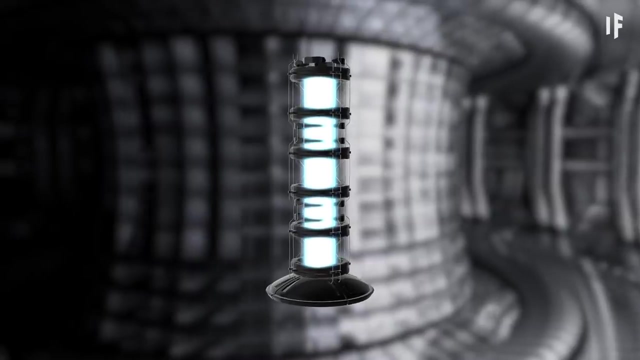 This is a spent nuclear fuel pool and you've just accidentally fallen into it. But what exactly is this thing? This large pool of water is meant to cool spent fuel rods after they come out of a nuclear reactor. While powering a nuclear reactor. 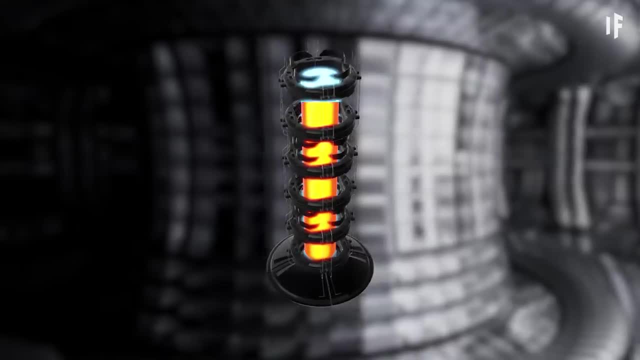 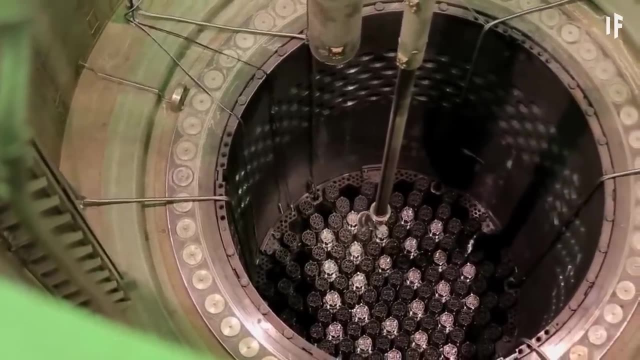 these fuel rods become very, very hot. We're talking 2,800 degrees. After it's spent three to six years inside of a nuclear reactor, a fuel rod is no longer efficient. Problem is it still emits plenty of harmful radiation. 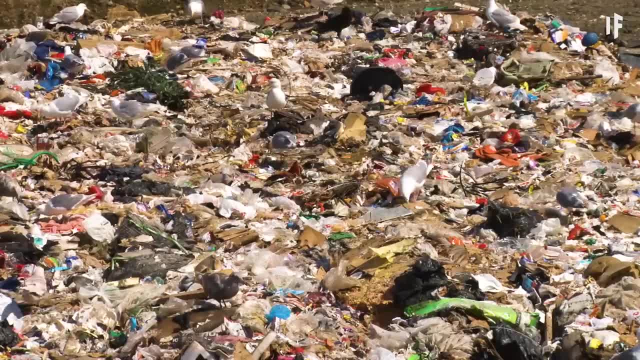 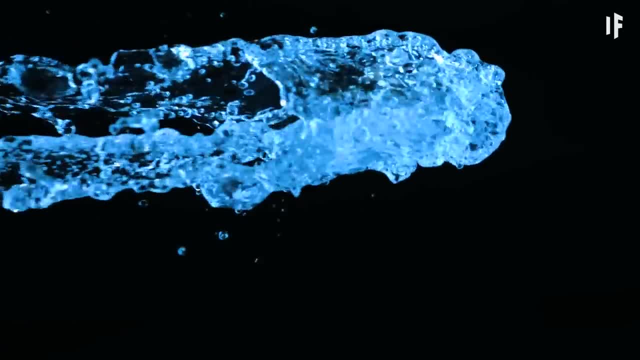 and it will for the next 10,000 years, Even though it's trash. there's not a garbage dump in the world that will accept it. So why is water a good place to put these things? Not only does the water spend several decades cooling the fuel rods, but it also affects their radiation. The water essentially acts as a biological shield, with hydrogen absorbing and deflecting the radiation bouncing against it. This makes it completely safe for you to stand near the pool with no ill effects. But what happens if you fall in the water? Well, as soon as you orient yourself, you'll quickly notice the temperature of the pool. This big tub of water won't be the refreshing dip you're looking for on a hot summer day. Instead, it'll be around 30 degrees, So a bit colder than your average hot tub. but still very warm, So a bit colder than your average hot tub. Let's hope you didn't accidentally turn off the water flow as you're falling into the pool. If you did, then you'd be in some serious trouble. Spent nuclear fuel pools are constantly cycling out water. 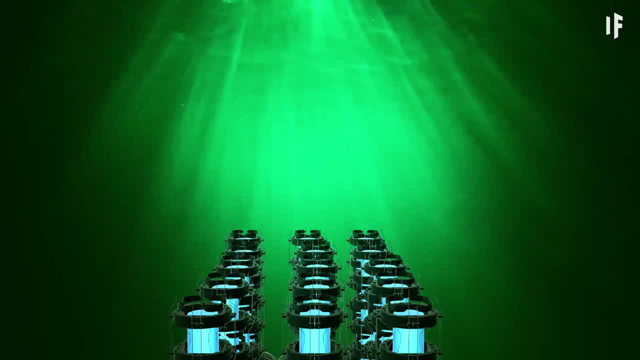 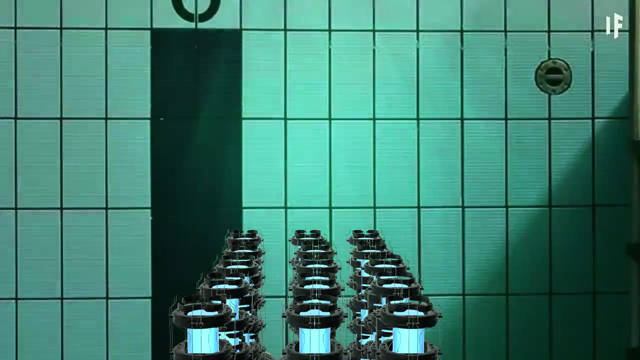 in order to keep it at a cool enough temperature. Remember, these fuel rods are incredibly hot and if the water isn't cycled out, then it would heat up significantly and slowly evaporate over time, resulting in you burning to a crisp. 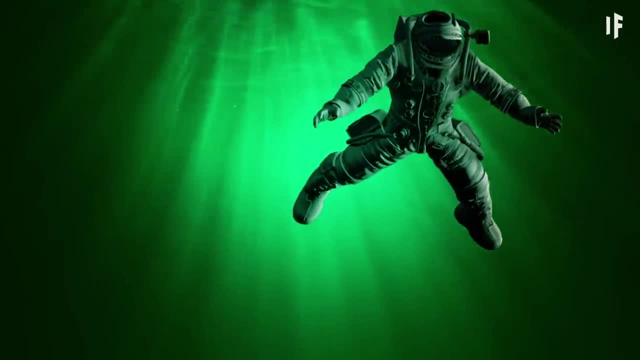 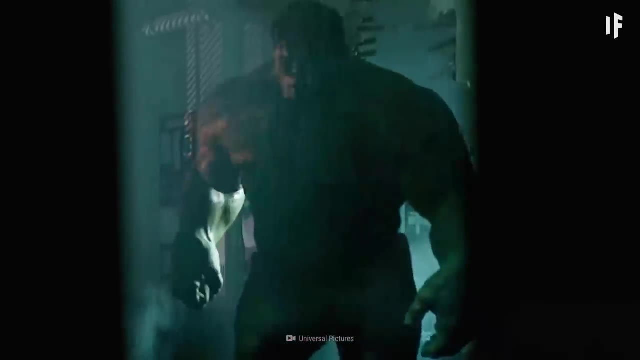 But that didn't happen. So now that you're starting to swim in this hot tub, So now that you're starting to swim in this hot tub or hot pool of water, when does the horrible radiation poisoning kick in? Or when do you turn green and start to gain superpowers? 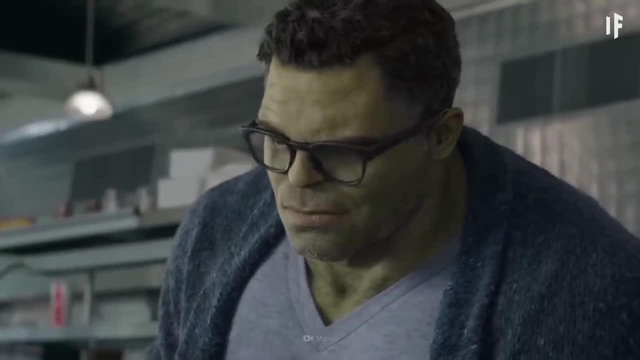 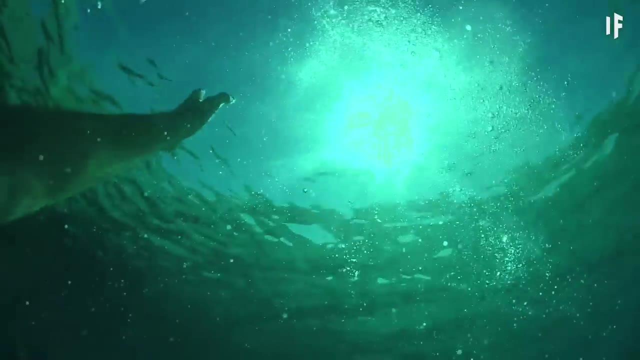 These are the sort of things that are supposed to happen when you fall into something that has nuclear fuel in it, right? Not exactly, Although that sounds like fun. it wouldn't happen to you if you fell into a spent nuclear fuel pool. That's because of the water.